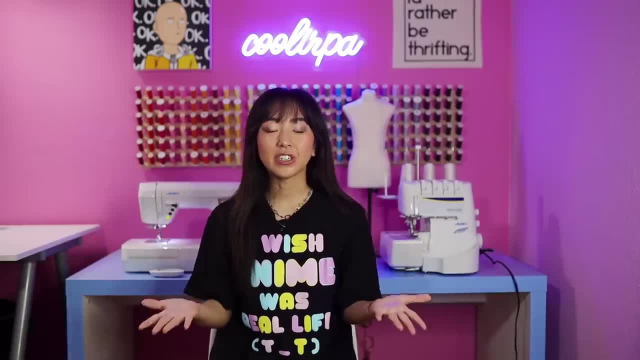 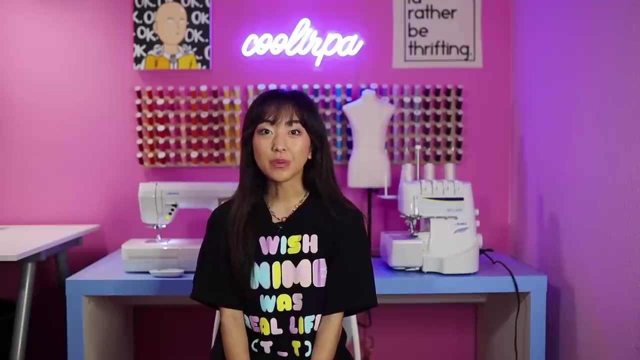 mistakes that beginners make- And I say beginners, but even experienced sewers make these mistakes as well. But if you are new to sewing, I hope that these tips will help you have a better learning experience And I hope that it saves you some time, fabric and money, because starting a new hobby can get expensive. I hope. 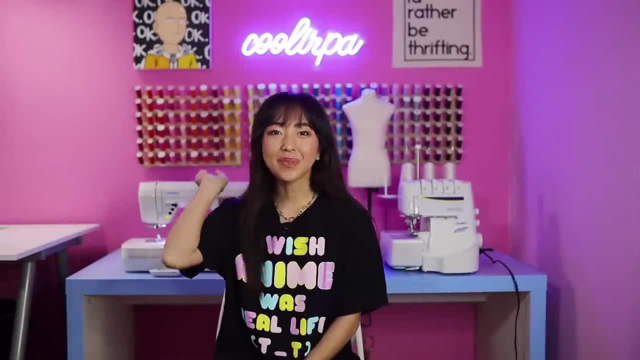 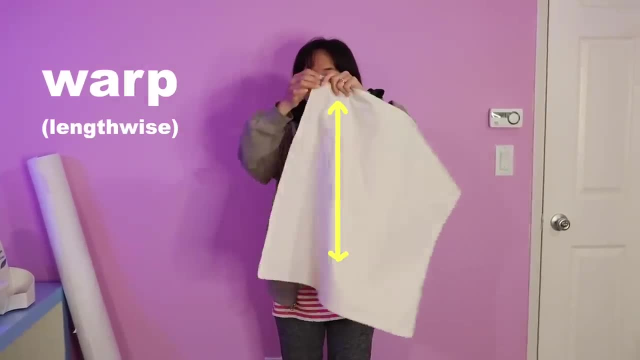 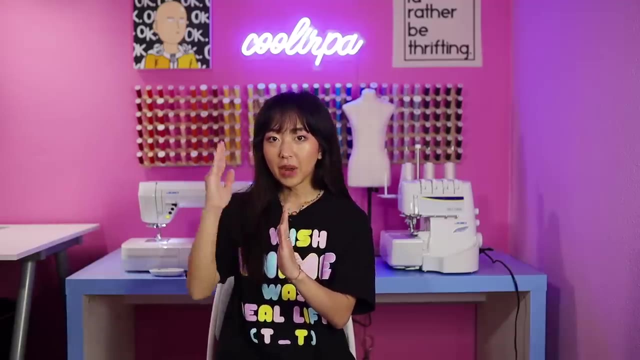 you enjoy this video and let's get started. Mistake number one: not cutting your pattern out on grain. So, on woven fabric, there is the warp, which is the lengthwise grain that goes up and down, And that grain line is parallel to the selvedge edge of the fabric. And then 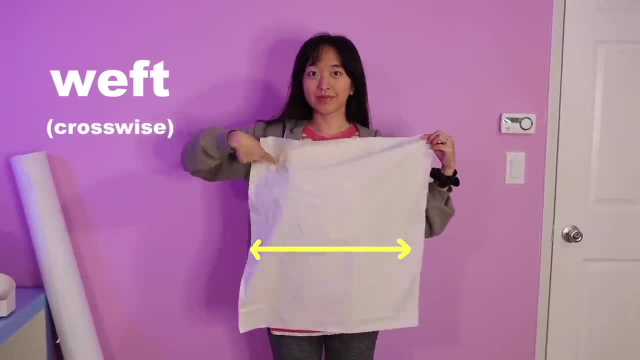 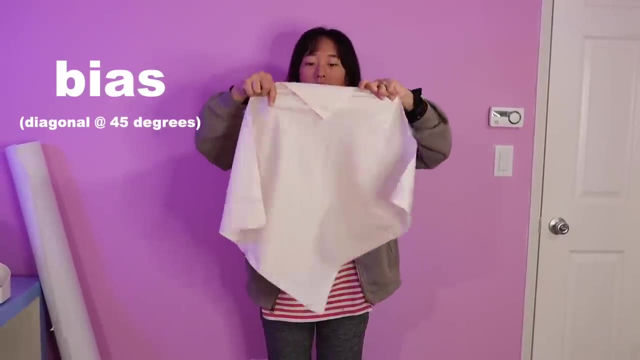 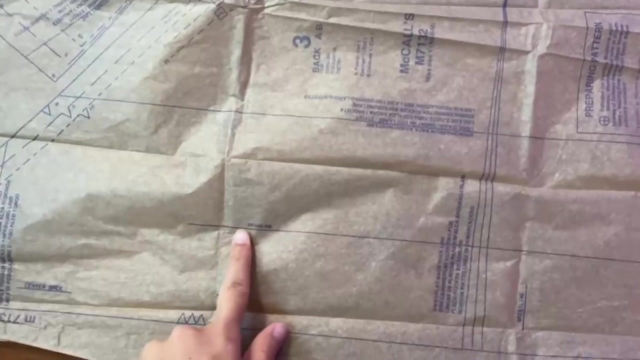 you have the crosswise grain that goes horizontal and that is called the weft. Then you have your bias, which goes diagonally across both of those And that will give you the most stretch and the most beautiful drape. If you're using a commercial pattern, normally it will tell you the grain line. 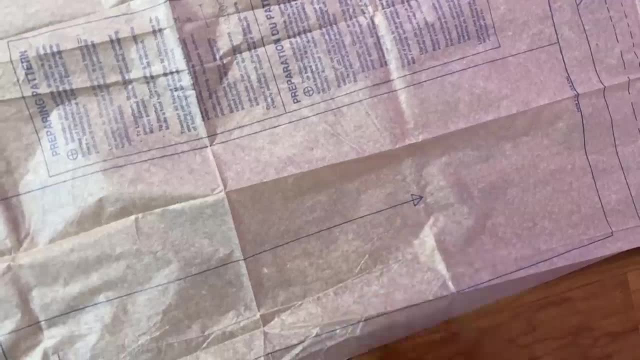 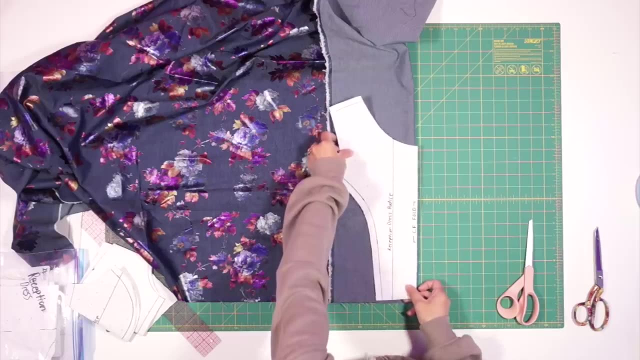 or if you are draping and creating your own pattern, you will be aware of where you put your grain line And then you would transfer that onto your fabric, And then you would transfer that onto your pattern. For example, here's a pattern I drafted And since the 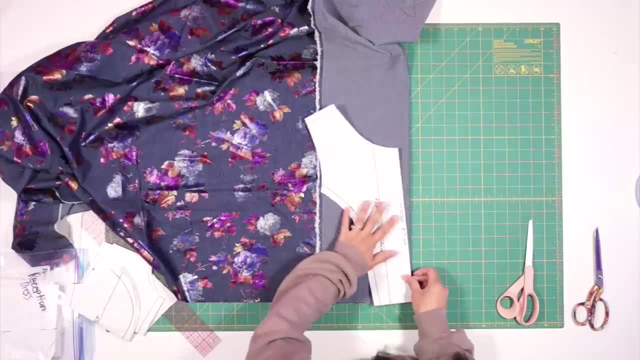 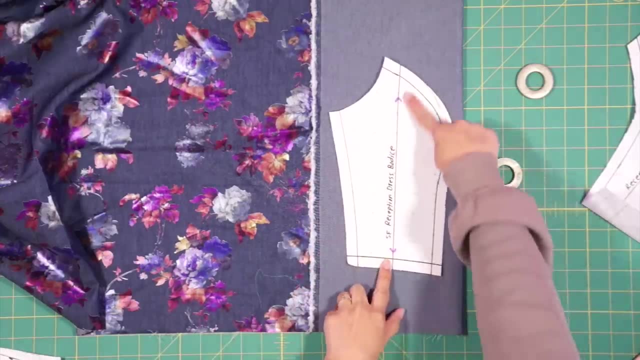 center front is cut on fold. the fold line is my grain line. The next pattern piece is not on fold and I marked a long arrow on my pattern indicating the grain line. You want to line the arrow with the selvedge edge or the lengthwise edge of your fabric and use. 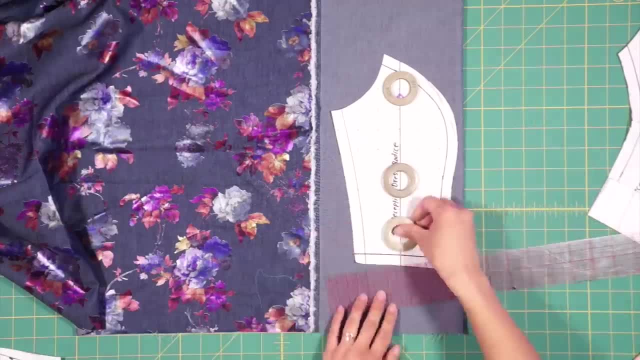 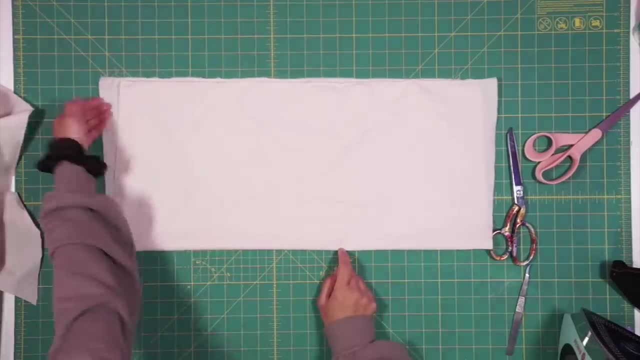 a ruler to make sure it's parallel all the way down. It's also important to make sure your fabric is on grain And you can tell by folding your fabric that it's parallel in half and matching up the corners. Before doing this, you should find the true warp. 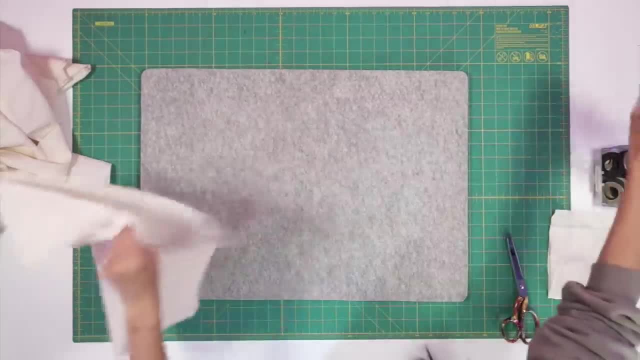 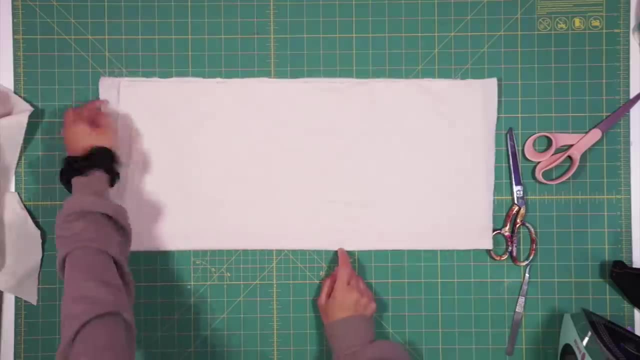 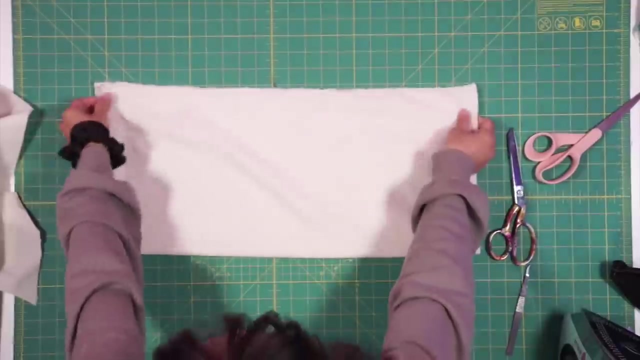 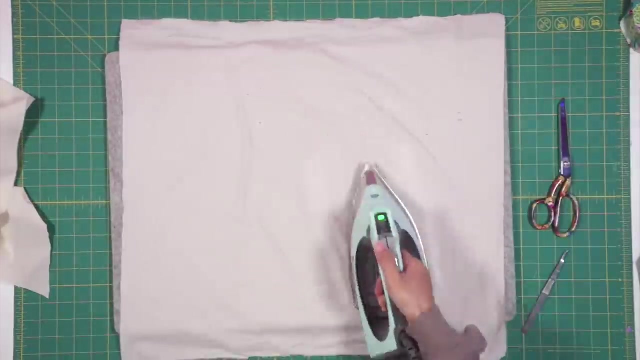 and weft so the corners are squared, and so you're not just following the uneven cutting from your scissors. If the corners are not matching up, grab the shorter corners and stretch the fabric diagonally until the grain line is straightened. In between, I like to 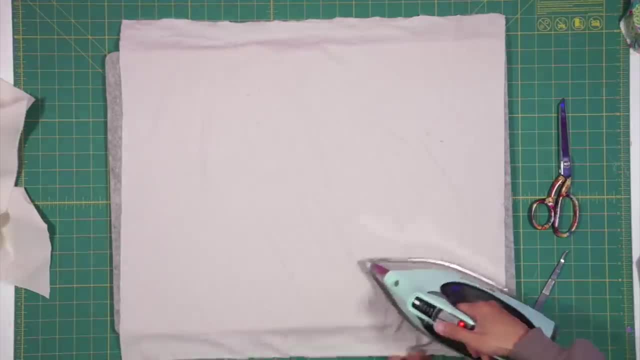 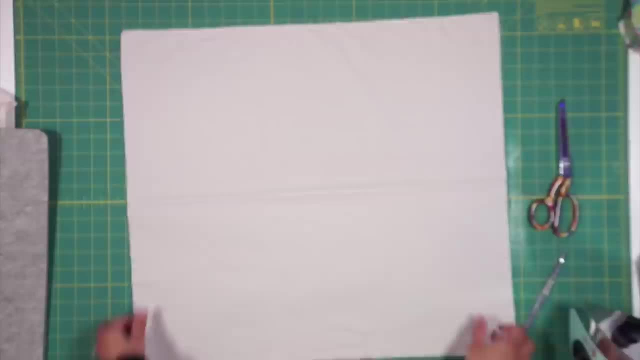 steam and gently press the fabric to help the grain stay in place. This process can take some time, so it's important to choose your fabric wisely so you're not working with anything too difficult. Mistake number two: Not ironing and pressing your seams after sewing, Pressing your project. 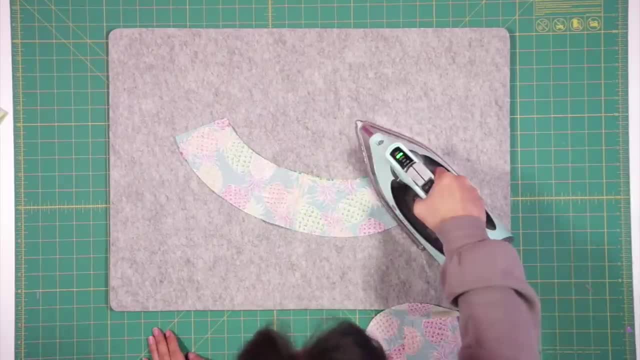 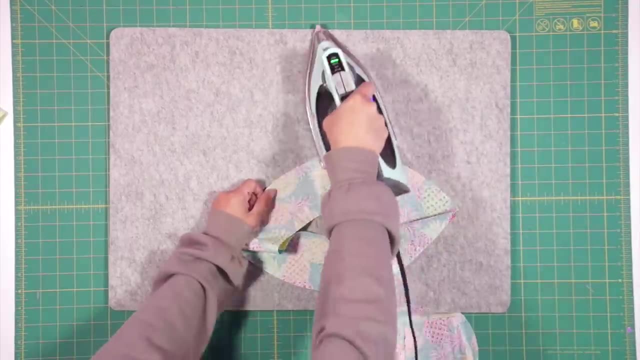 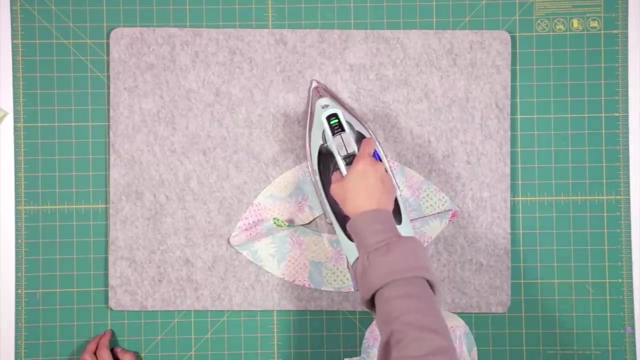 before sewing. the next step is going to help your seams lay more flat and allow for more accurate sewing, And overall it's going to give a very professional look, even if your sewing wasn't perfect. PS. Check out my new wool ironing mat. Since my room is smaller, I got rid of my ironing. 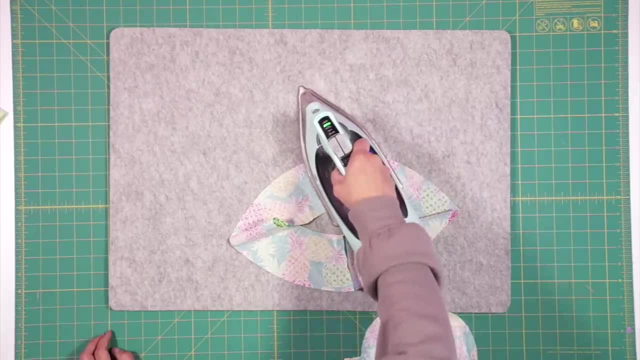 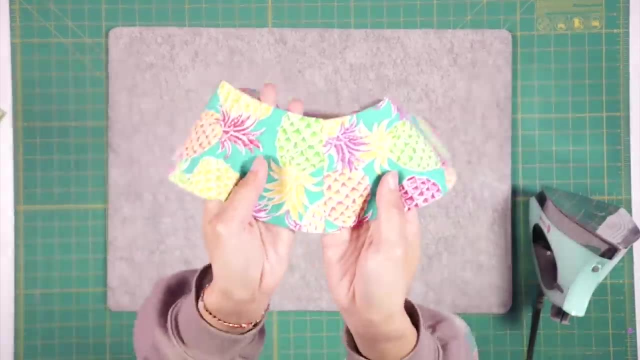 board to save space, and now I can film my pressing on the tabletop. When I use steam on this mat, though it does smell like sheep or the goats that our neighbors have, So if you're sensitive to smell, I don't recommend it. But honestly, it's so useful and saves. 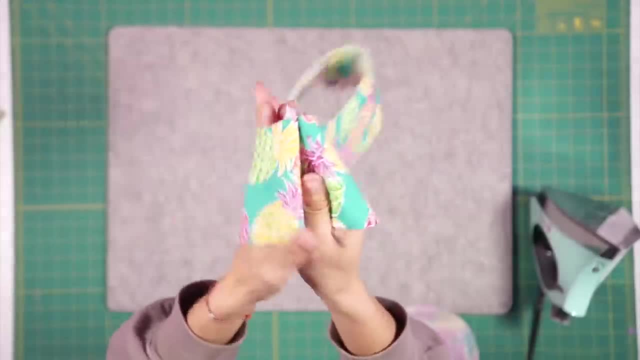 lots of space. Link will be below in my description box if you want to check it out. I also learned that pressing your seams allows the thread to melt away. So if you want to add more thread, you can press the button on the top of your fabric to make the seam. 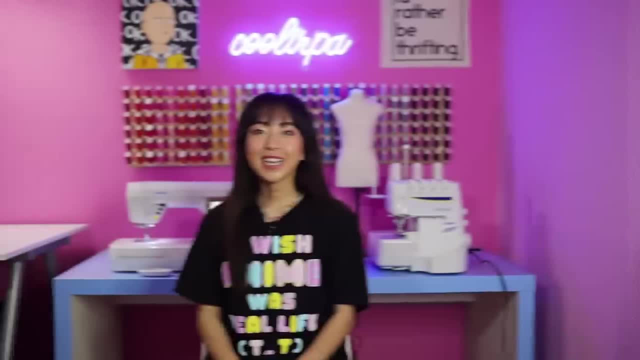 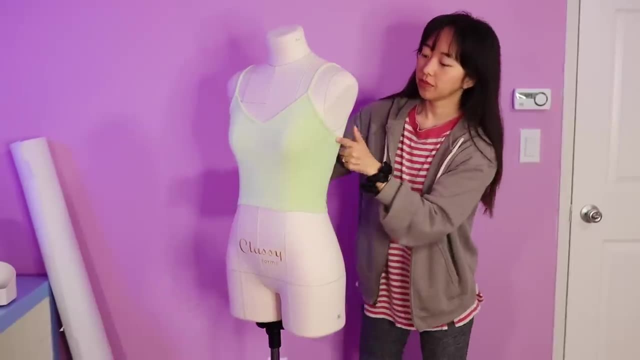 a lot stronger and give it a more finished look. Mistake number three: Forgetting to add seam allowance, so your garment ends up being too small and tight. If this is the top, I want to recreate and sew The seam line when I'm 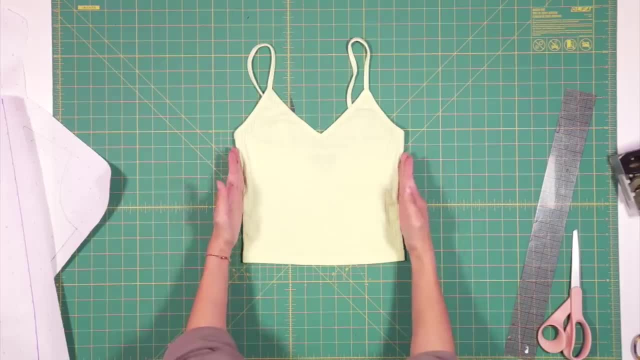 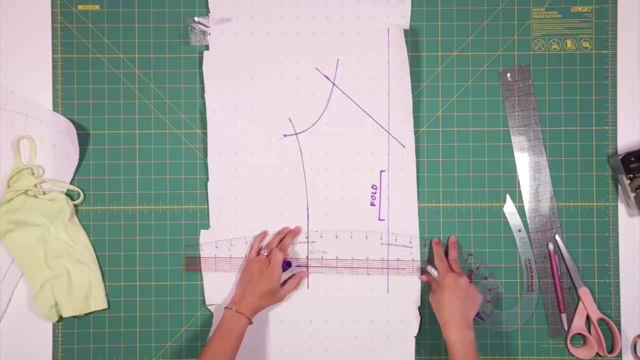 sewing. it is here, But if I don't add seam allowance and just trace it as is, my seam line will actually move in more and I'll be sewing it smaller. So if you want your clothes to fit you properly, make sure to add seam allowance along your fabric. 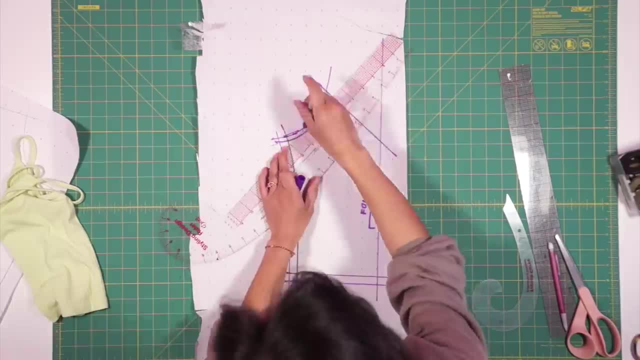 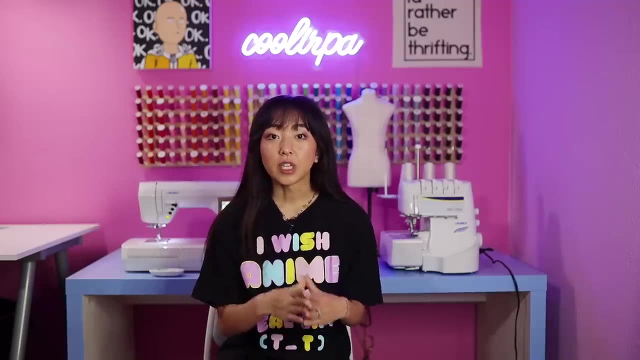 I normally add a half inch seam allowance on all of my patterns, but it really depends on where the seam allowance is being placed. If you are unsure or making it for someone else, it's best to always give yourself a bigger seam allowance, so there's room for. 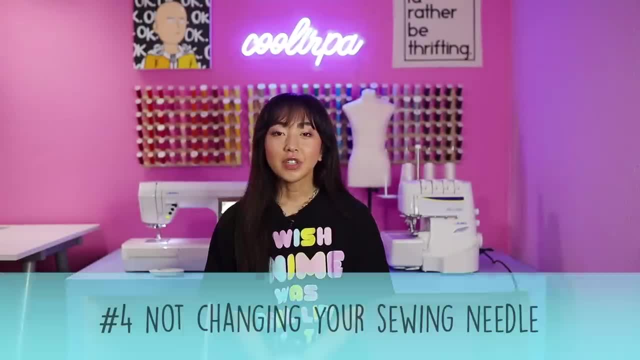 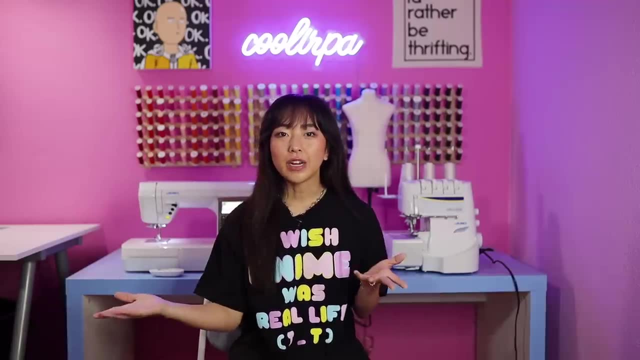 adjustment. Mistake number four: Using the wrong needle for the fabric type you're working with. I do think the problem is also not knowing what fabric you're working with. If that's something you struggle with, this book Textile PE is going to help you out a lot. So if you're 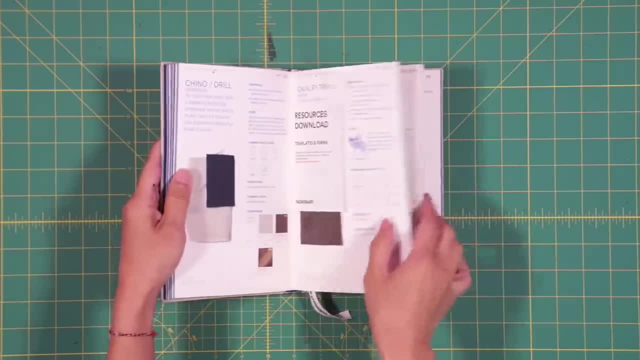 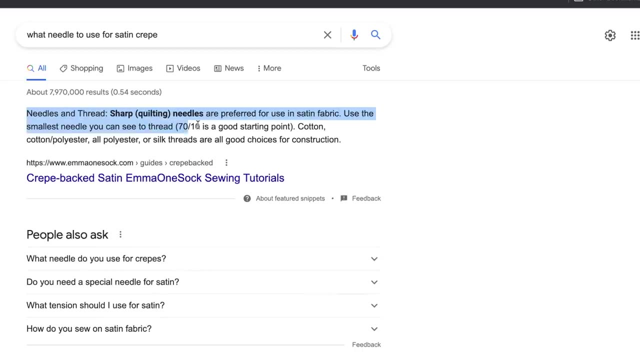 interested in learning more about sewing, please check out the link in the description box. I'll link it below along with my 10% off code for anyone interested. Once you do know, you can do a quick Google search to learn what size and type needle. 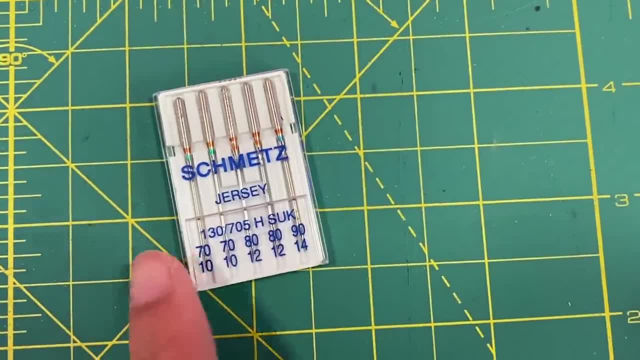 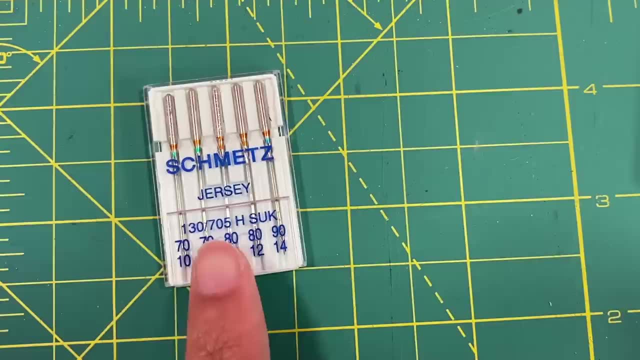 to use. I also want to share what the numbers on the needle packs mean because it looks confusing. but basically, the higher the number, the thicker and heavier fabric you can sew, And the lower the number is the finer the needle and the more lightweight fabric you can sew. It's. 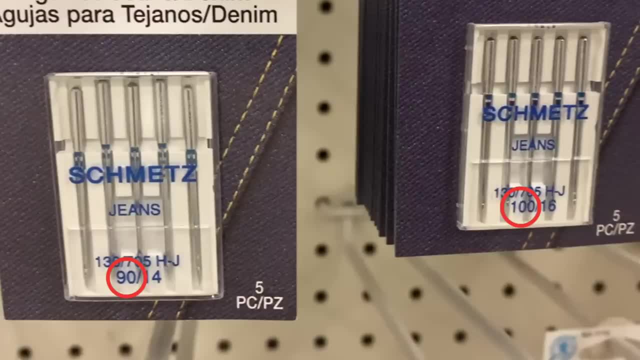 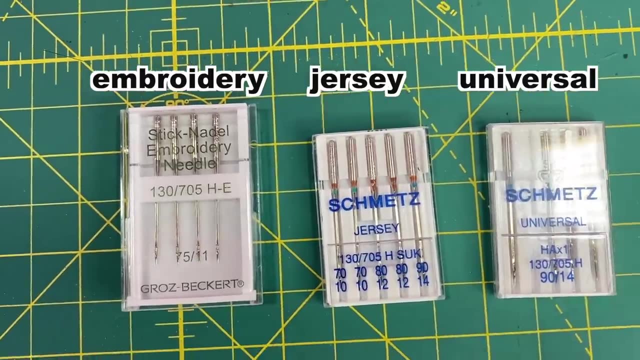 confusing because there's two numbers. but the bigger number is the heavier fabric you can sew. The bigger number is just in European size and the smaller number is in US size. Not only is the needle size important, the needle type is as well, because there's different. 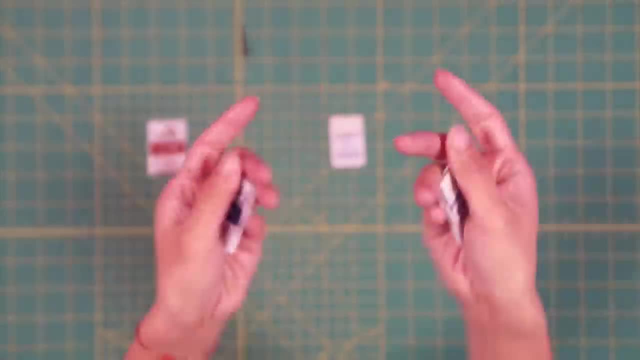 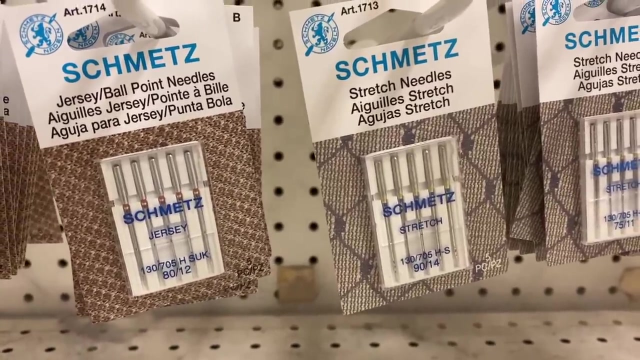 types of fabric, like woven knits and leather, that you might be working with. For example, when I sew stretch fabric, I make sure to use a jersey or ballpoint needle, because the tip isn't as sharp, It's more rounded, so it doesn't tear the fabric or break the elasticity. 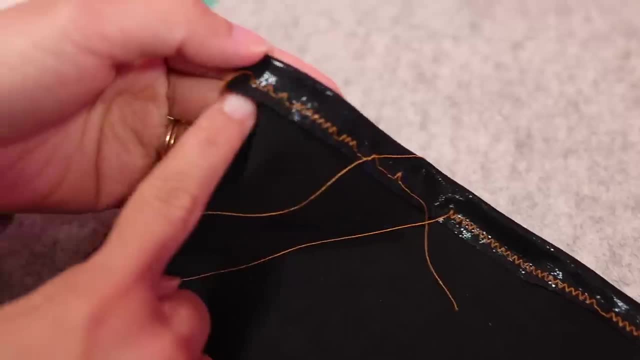 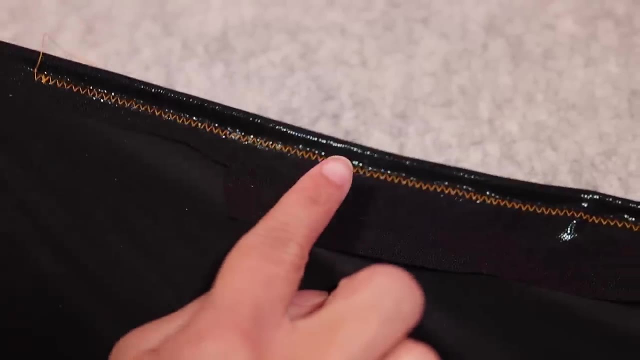 Here I was using the right needle type, but the stitches were still skipping, so I'm going to have to also change the needle size to a higher number, and then it's sewed properly. Lastly, make sure you use the right size thread for your needle size. You don't want to be 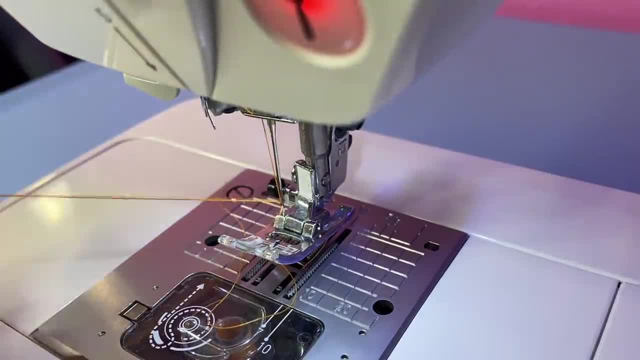 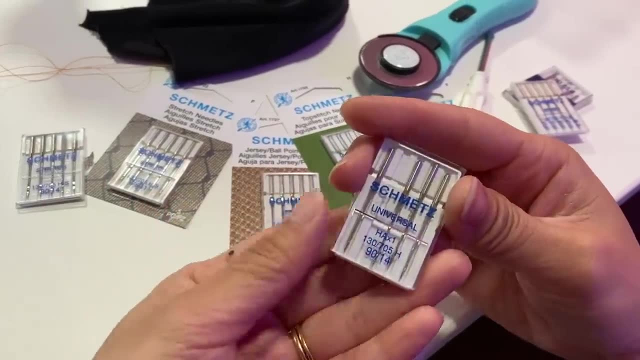 shoving a heavy thread into a fine needle, because that will cause problems with your sewing as well. My problem with having a bunch of different size needles around is that if you don't put it back then you kinda forget the thread. I think this is a good thing, but you could 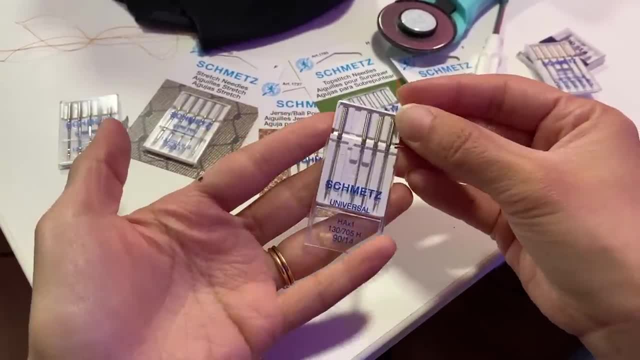 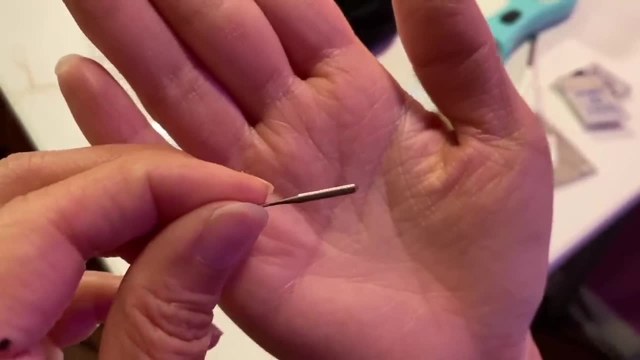 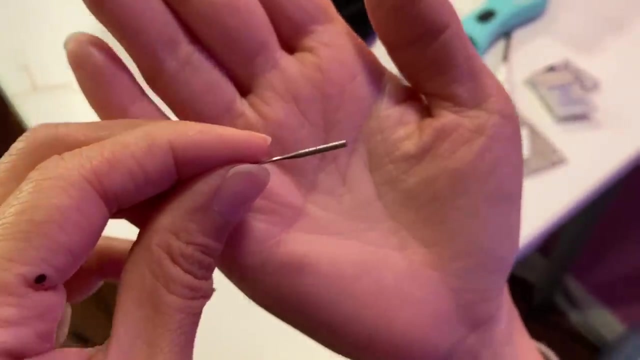 also be able to do something like this. I feel like I have the perfect amount of fabric so I can sew this around. before I sew, forget what needle it is, but the size of the needle is actually engraved on top. it's just super hard to see. but you need a- what is it called? a magnifying glass? that's what it's called you. 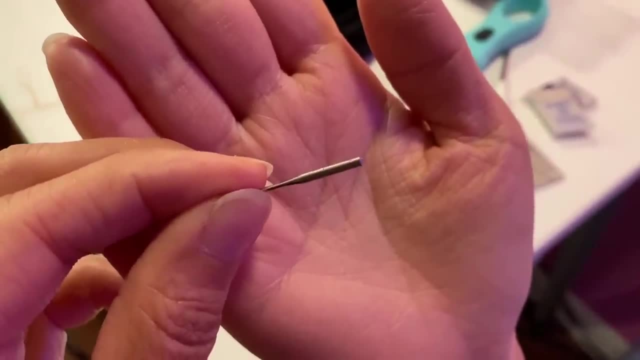 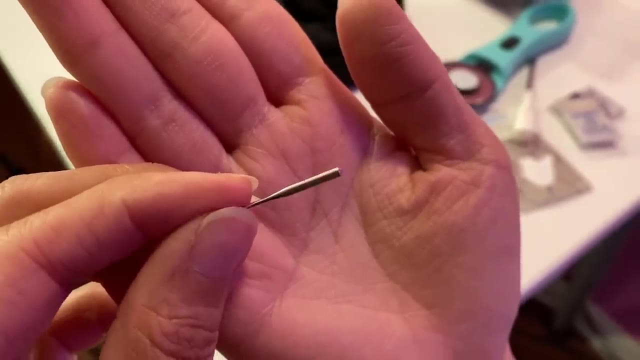 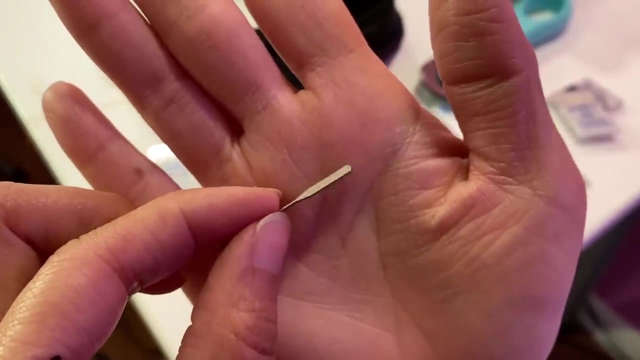 would need a magnifying glass to see the number, but if i squint really hard or hold it in the right light, i can sometimes see it. um, so if you also, you know, misplace your needle or forgot what size it is or what it's meant for, you can try looking there. mistake number five: choosing the. 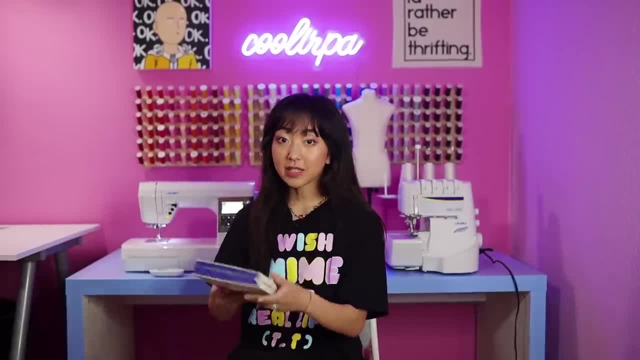 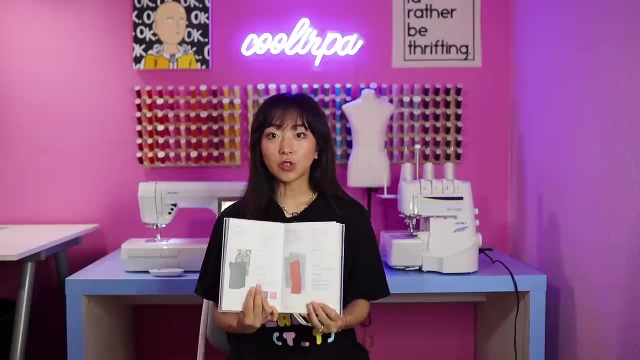 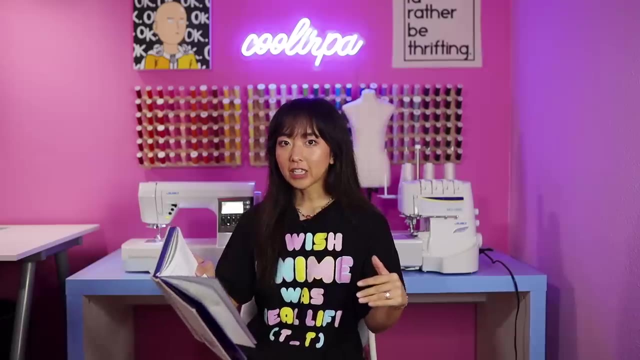 wrong fabric for the project you're making. again, the book textilepedia would be super helpful if this is something you struggle with. so here i flipped it to chiffon and under that it gives a description of like the properties and the common things that people make out of chiffon. so it says: 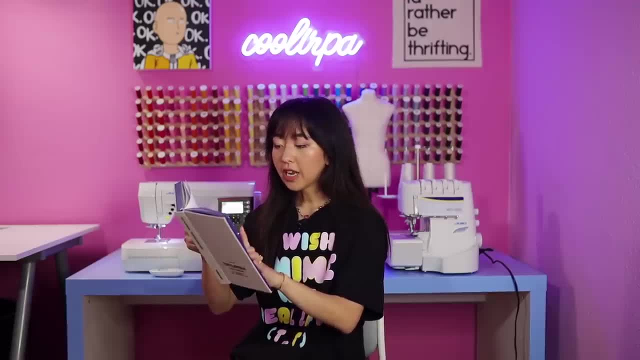 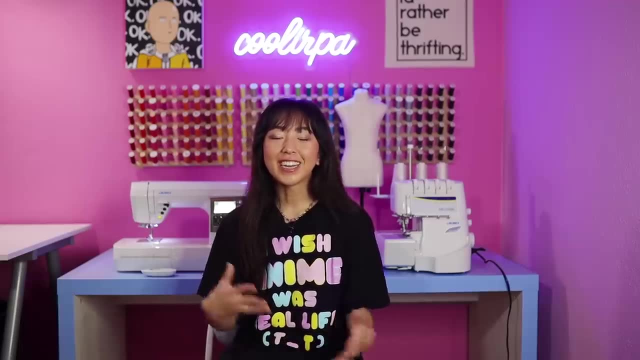 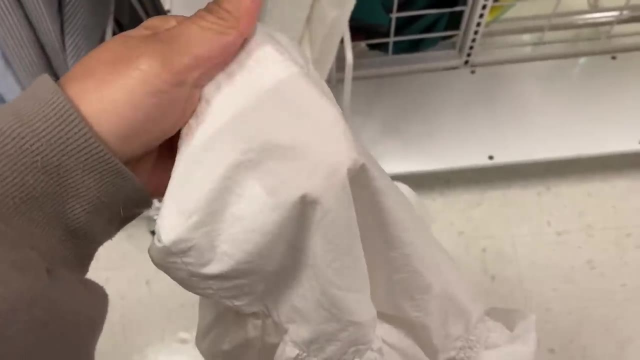 blouses, scarves, lingerie, gowns, bridal wear and embroidery. for me, because i've been sewing for so long and i study a lot of the clothes in my closet, i can kind of tell what material would work well for a blouse or for bottoms, if there's something similar in your closet that you can. 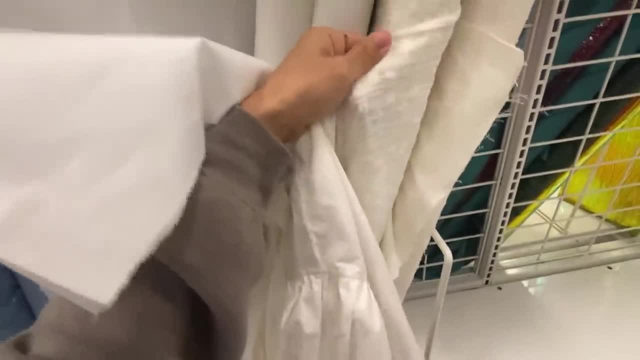 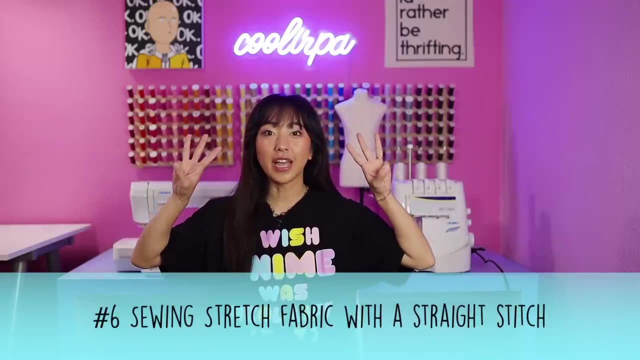 bring fabric shopping with you. that would be really helpful as well. that way you can compare. you can compare the fabric shopping with the fabric shopping with you. that would be really helpful as well. that way you can compare the two in person. mistake number six: sewing stretch fabric with a straight stitch. this was a mistake i made, as well as a beginner, and for some reason, 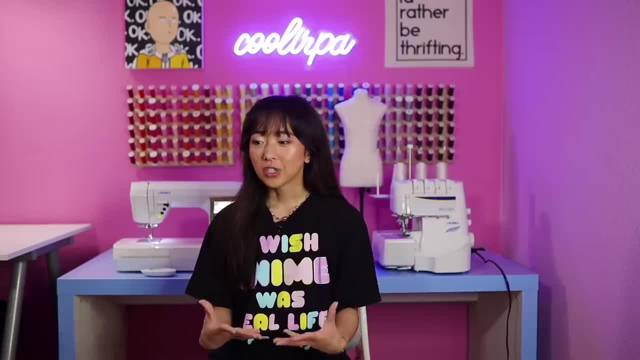 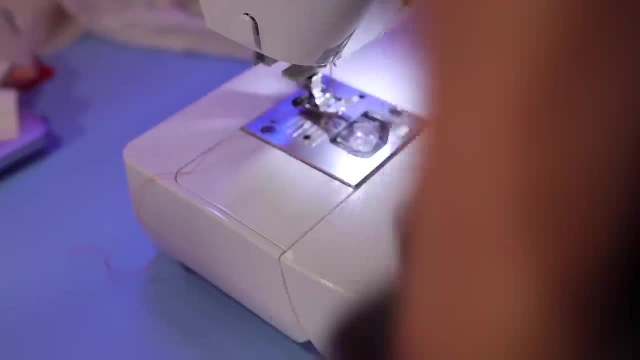 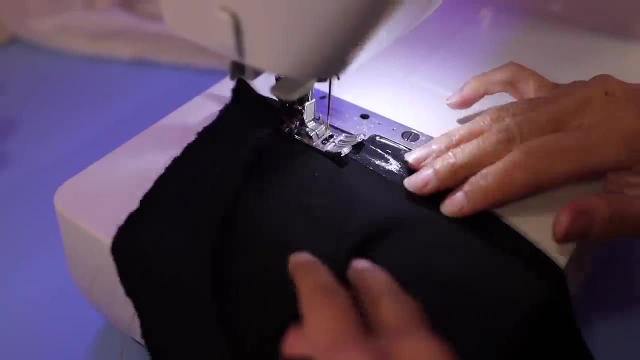 when we're learning how to sew, beginners are just more drawn towards stretchy fabric, and i think that's because we don't want to sew a zipper. the problem with sewing a straight stitch, straight stitch- on stretch fabric is that it doesn't stretch the fabric and it doesn't stretch the fabric. 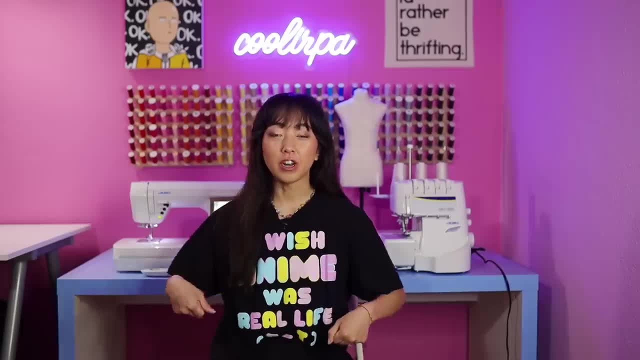 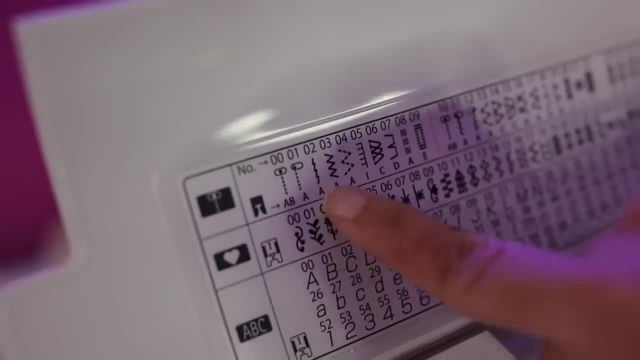 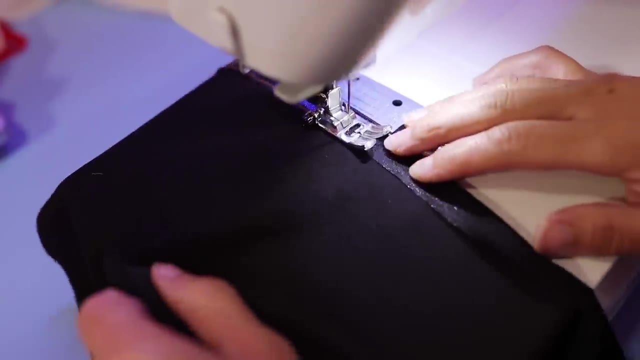 stretch with the fabric. so what happens when you try to put it on the seam pops? listen to this: a better stitch to use if you have it on your machine is the stretch stitch, or aka lightning stitch, and this stitch, basically is a zigzag stitch. that is very 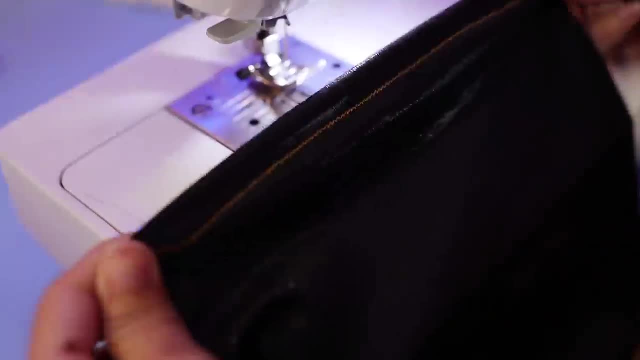 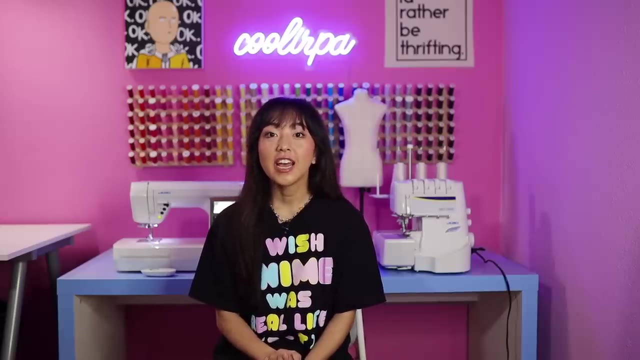 narrow so it looks like you're sewing a straight stitch, but it's not so. it allows the stretching of the fabric. still, if you do not have this stitch setting on your machine, a zigzag stitch will work fine as well. and as you get more experience with sewing and 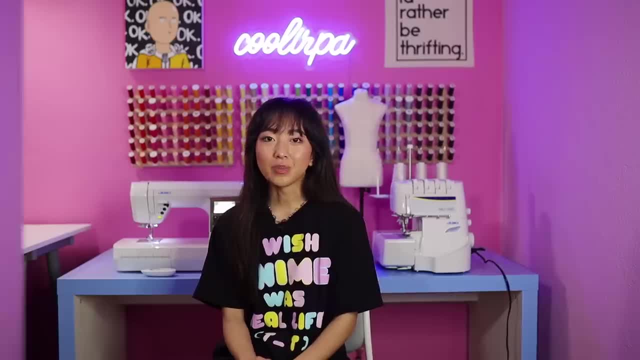 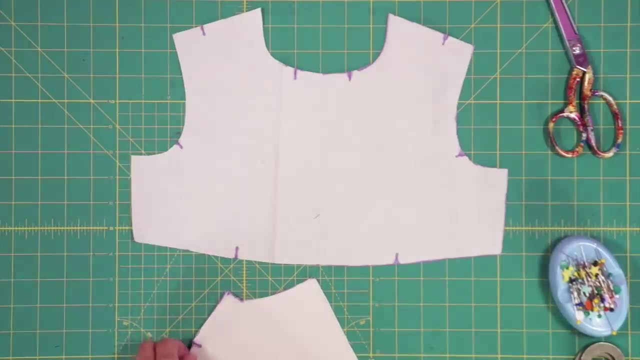 want to invest in a serger. that would be my number one option. mistake number seven: not pinning and notching your fabric before sewing. when we're doing a lot of diy sewing at home, we want to do things quickly, so we'll skip pinning and notching our fabric, but it actually saves. 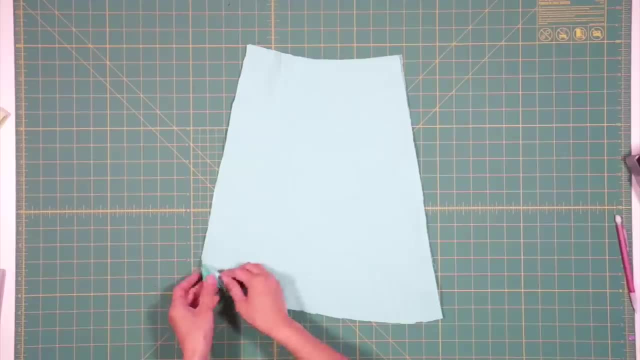 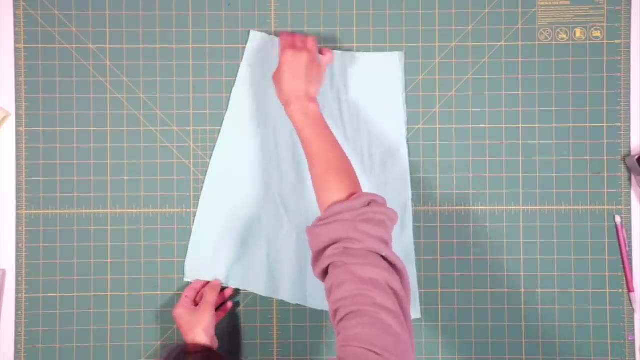 you some trouble down the road if you take the time to do so. when i don't notch and pin my pieces together once i'm done with my sewing and i'm ready to go to the next step, i'm going to cut them exactly the same. if i know i'm working with simple fabric that won't move, i can skip.